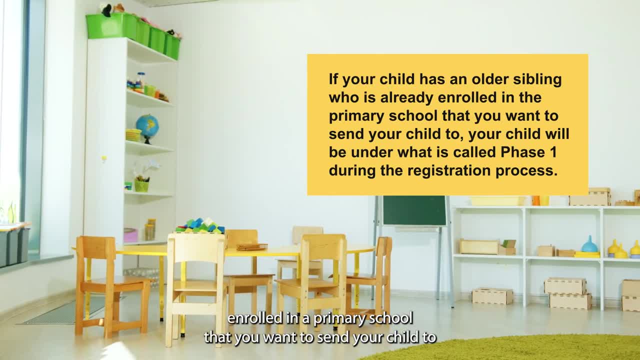 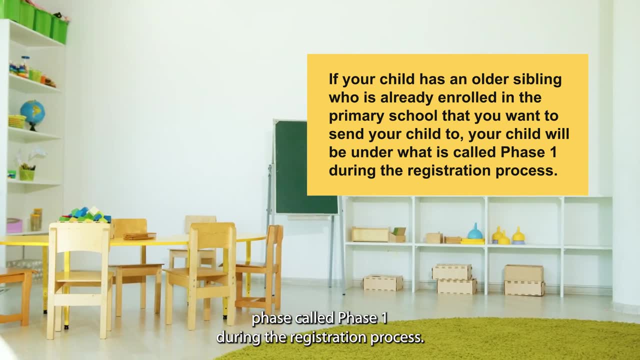 an older sibling who is already enrolled in a primary school that you want to send your child to. your child will be under phase 1 during the registration process. This means your child will be given priority over other students who do not have a primary school registration名. EssexSC. 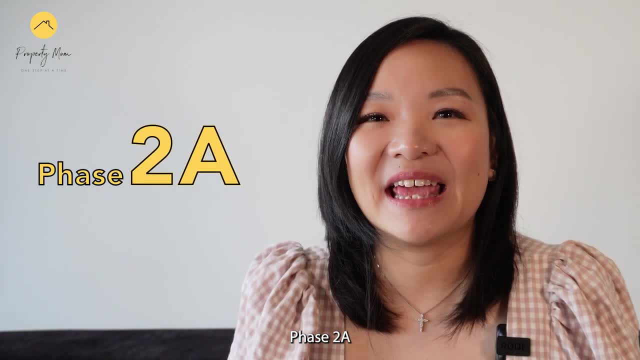 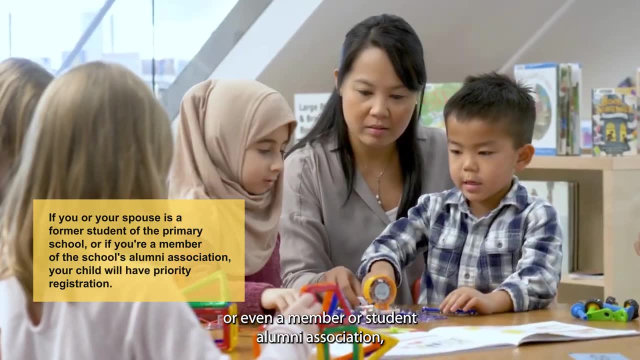 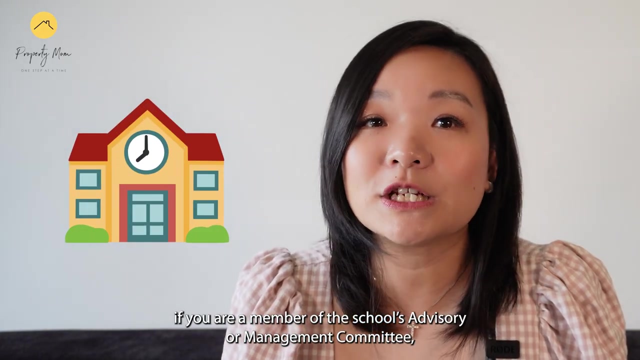 a sibling already attending the school Phase 2A. if you or your spouse is a former student of a primary school or if you are member of student alumni association, your child will have priority registration And second, if you are member of the school advisory or management committee, your child 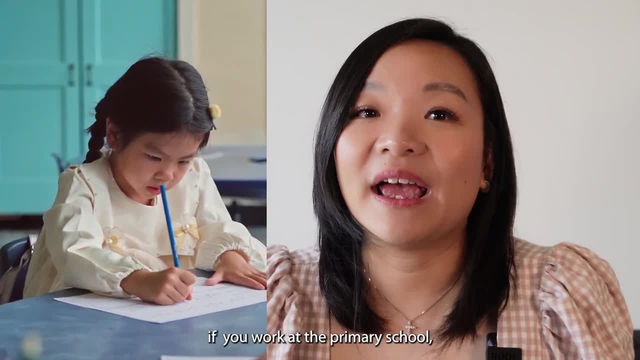 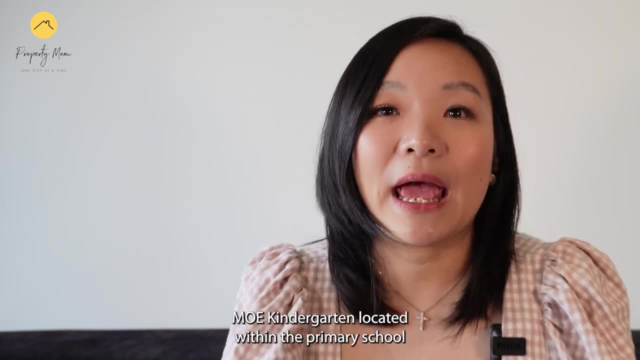 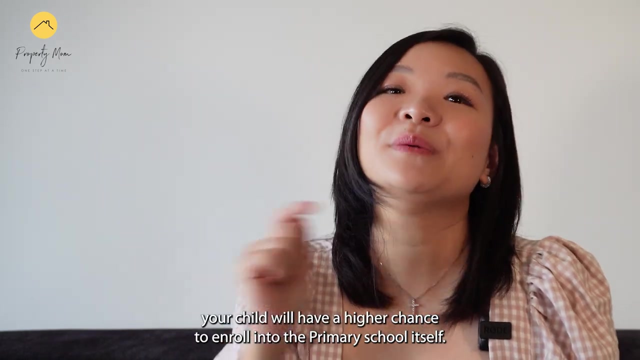 will also have priority. Thirdly, if you work at a primary school, your child will have priority over other students. Finally, if your child is currently enrolled in a MOE kindergarten located within the primary school, your child will have a higher chance to enroll into the primary school itself. 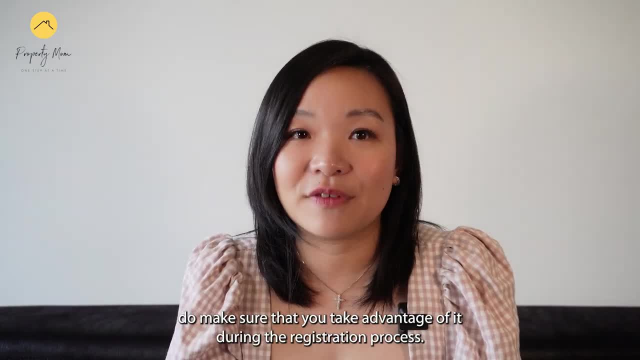 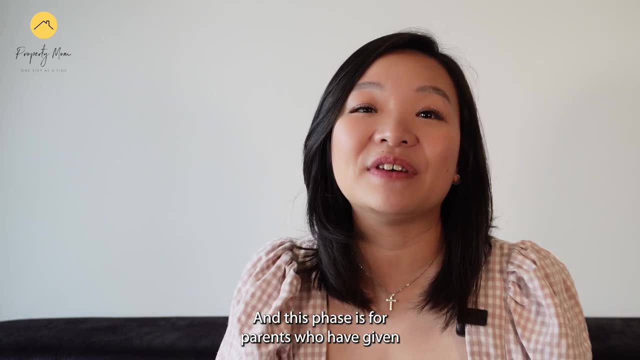 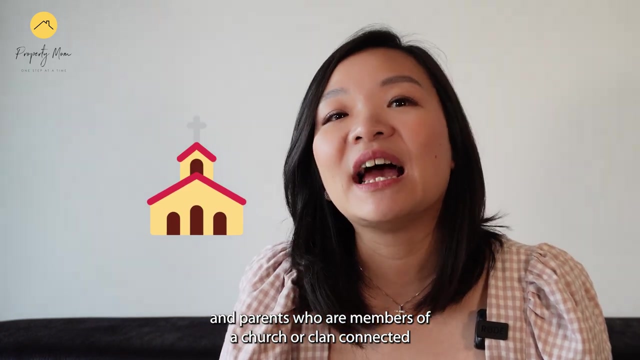 So if you meet any of these criteria, do make sure that you take advantage of it during registration process. Phase 2B- and this phase is for parents who have given at least 40 hours of voluntary service to the school and parents who are members of church or clan connected to the- 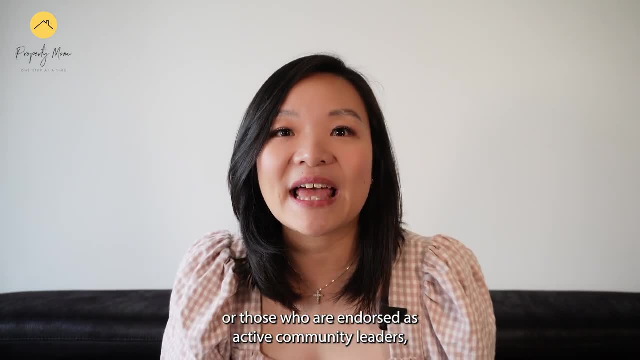 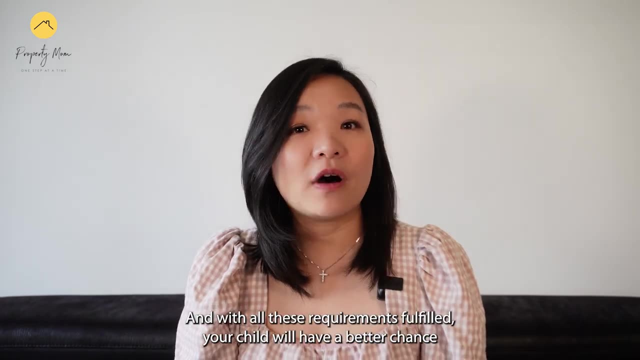 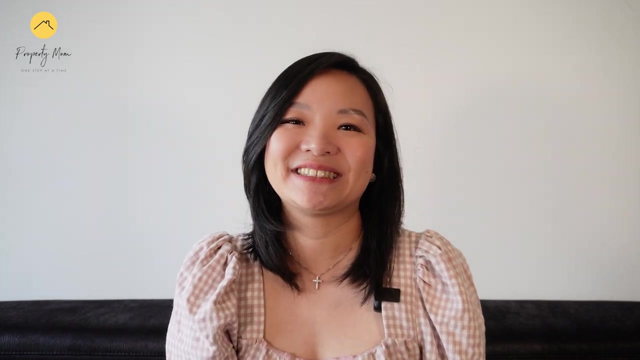 primary school or those who are endorsed as active community leaders may also be eligible for this category And with all these requirements fulfilled, your child will have a better chance of getting into the primary school of their choice. So right now we are at Phase 2C, and if your child does not get a place in an earlier phase, 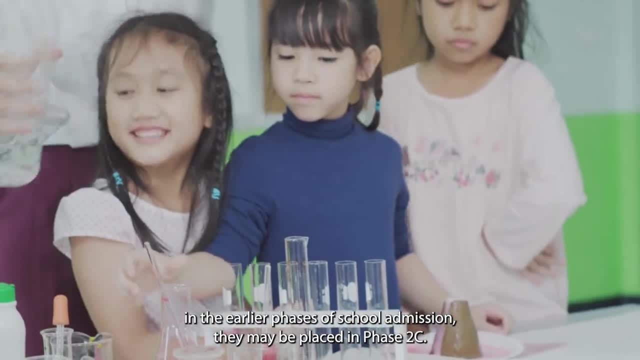 of the school admission. they will be placed in Phase 2C For children in this phase of the school admission. they will be placed in Phase 2C. For children in this phase. they will be placed in Phase 2C. 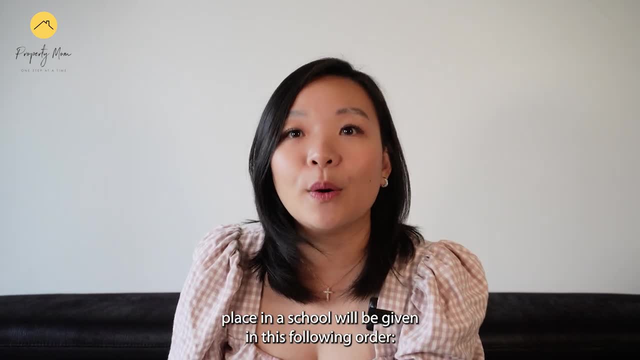 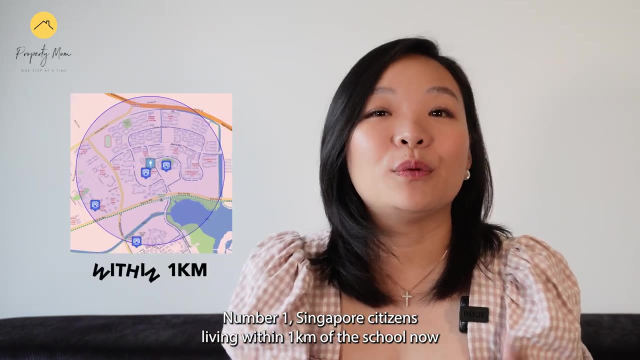 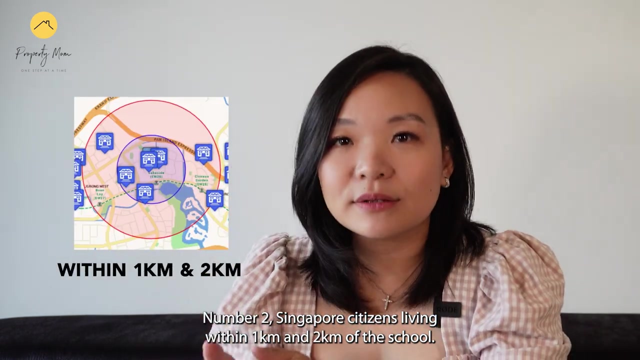 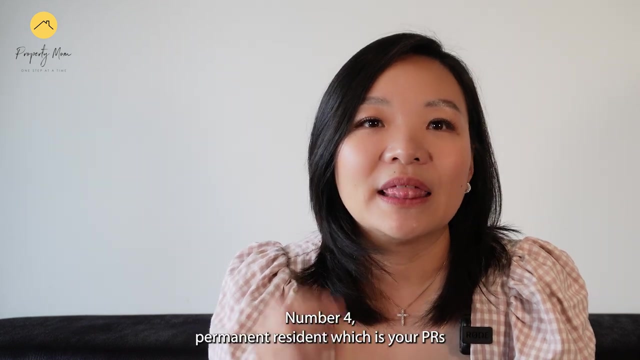 The priority admission to primary 1 place in a school will be given in this following order: 1- Singapore citizen living within 1 km of the school. 2- Singapore citizen living within 1 km and 2 km of the school. 3- Singapore citizen living outside 2 km of the school. 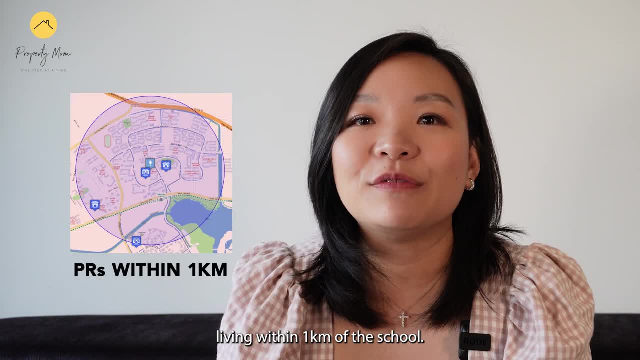 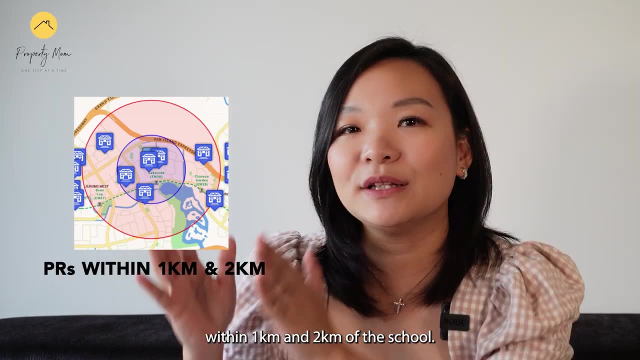 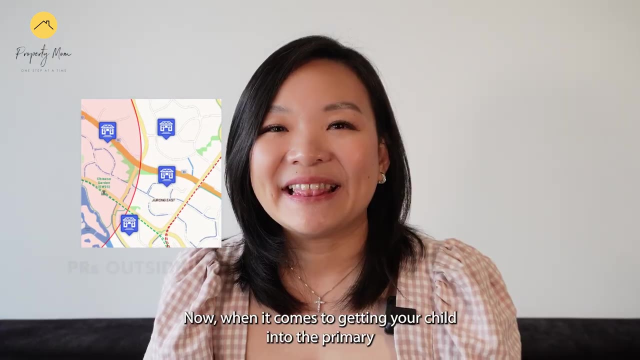 4- Permanent resident living within 1km of the school of the school. number five will be your pr living within 1 km and 2 km of the school and, lastly, will be pr living outside 2 km of the school. now, when it comes to getting your child into the primary, 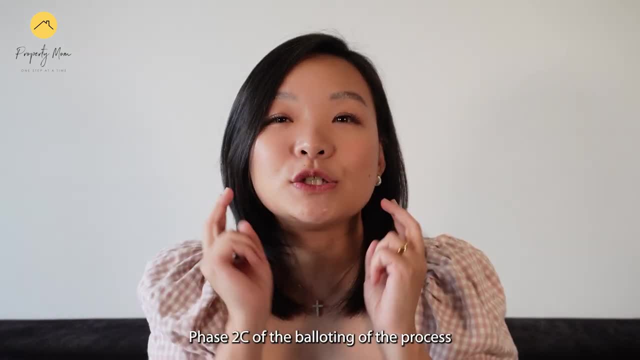 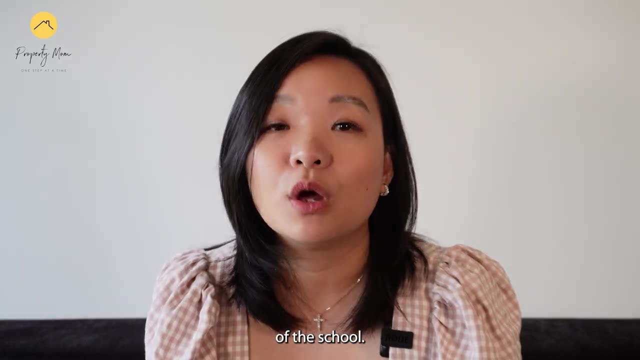 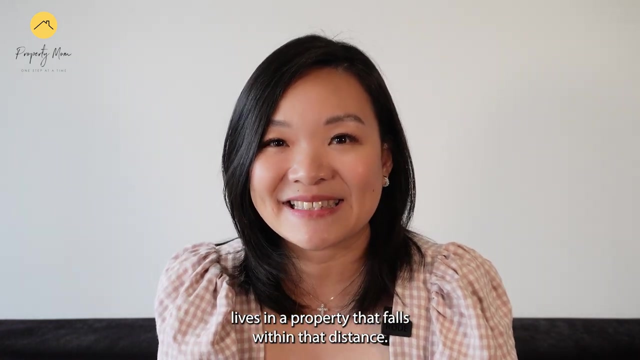 school of your choice. it pays to be prepared. phase 2c of the balloting of the process give priority to children who lives within 1 km of the school. so one way to increase your chance is to make sure that your child live in a property that falls within that distance, if you don't already own a. 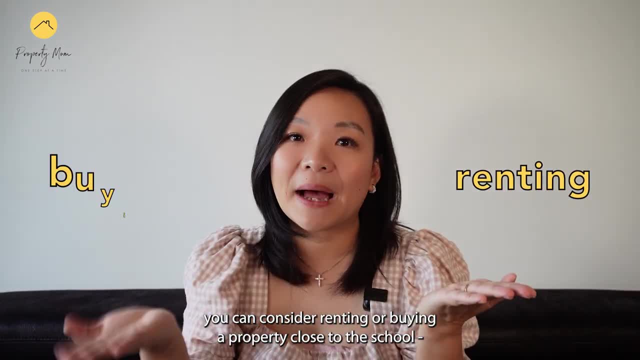 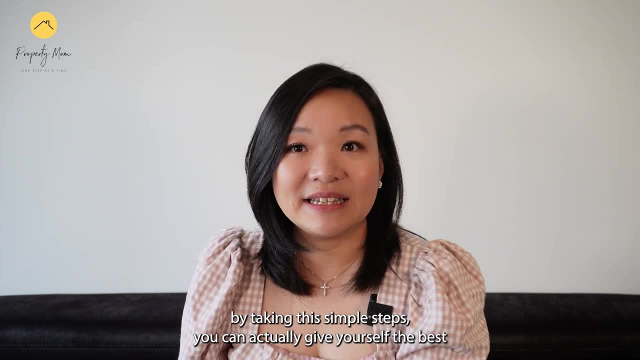 place near your preferred school. you can consider renting or buying a property close to the school just to make sure that you stay in the address for at least 30 months. by taking these simple steps, you can actually give yourself the best possible chance of securing a place for your chosen. 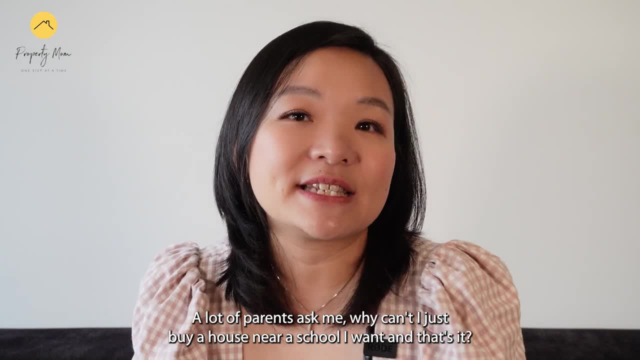 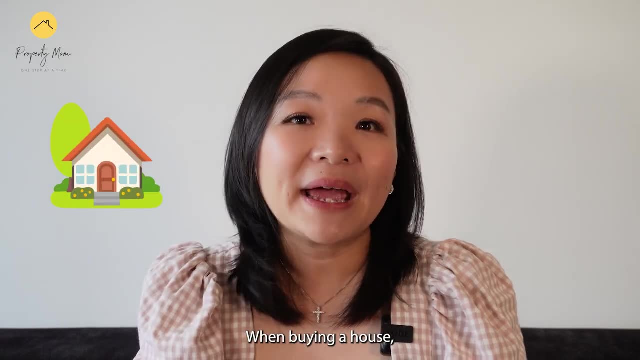 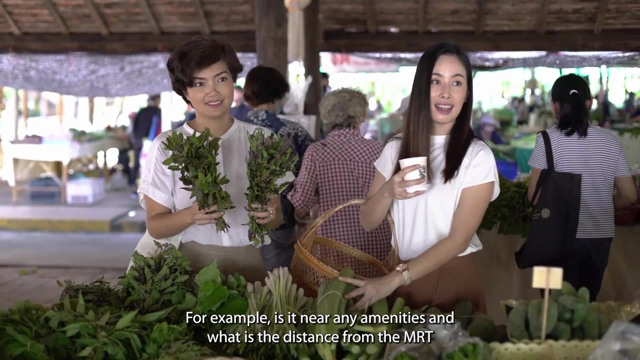 primary school. a lot of parents ask me: why can't i just buy a house near a school that i want and that's it? yes, that is correct to a certain extent. when buying a house, there's a lot of things to consider. for example, is it near any amenities and what is the distance from the MRT? and also 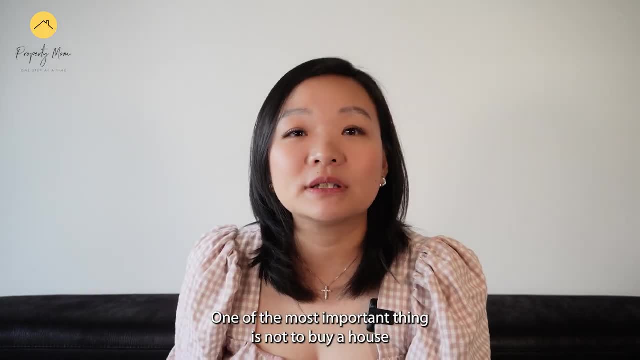 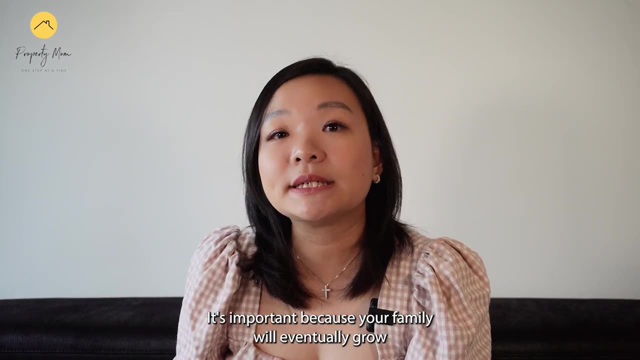 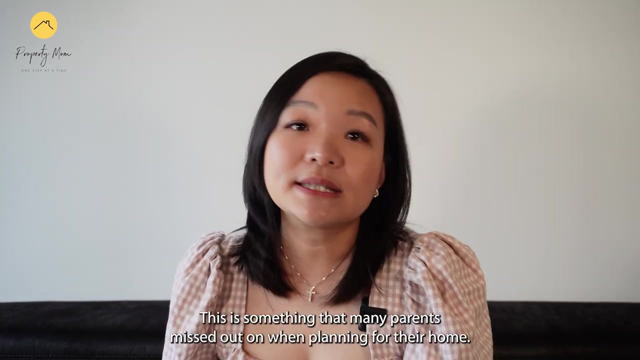 is there any growth potential? one of the most important thing is not to buy a house that will lose money in an event that you want to sell. it is important because your family will eventually grow and you will likely need to change to a bigger house later. that is something that many parents miss out on when planning their home. they fail to do their 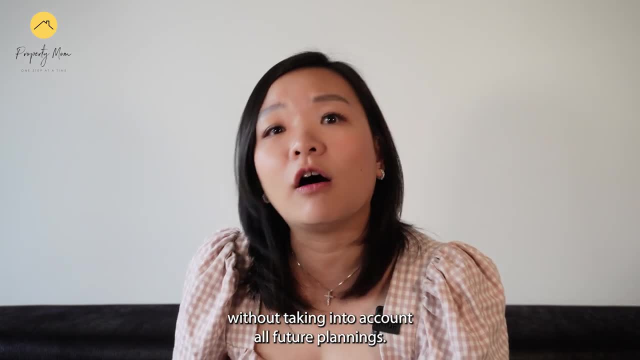 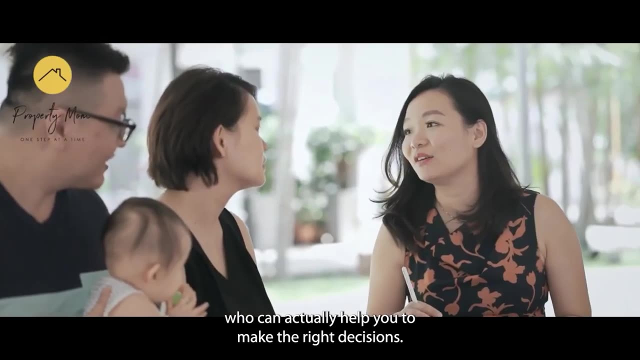 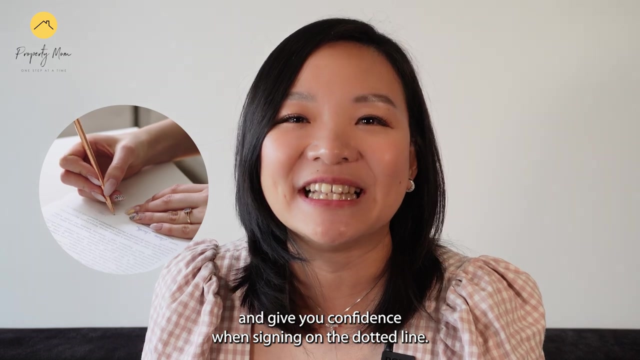 research and rushed into buying a property without taking into account all future plannings. this is why it's important to consult with professionals who can actually help you to make the right decision. with their help, you'll be able to find a property that fits your needs and gives 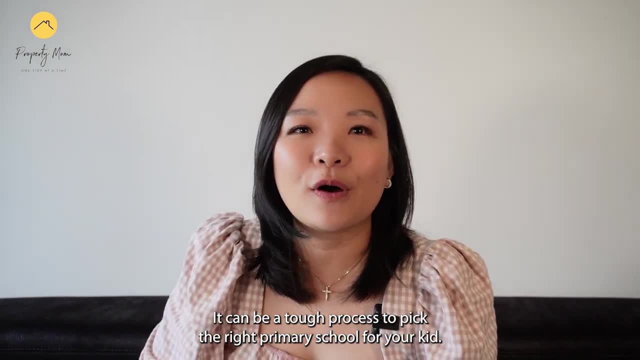 you confidence when signing on the dotted line. it can be a tough process to pick the right primary school for your kid. i hope this video will give you confidence when signing on to Doct 343 on the dotted line. it can be a tough process to pick the right primary school for your kid. i hope this video will help you sign up bsy408. 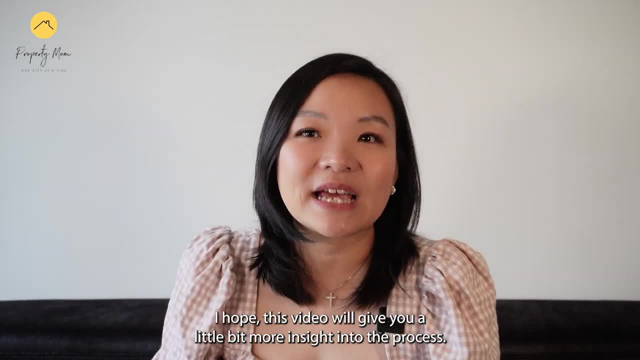 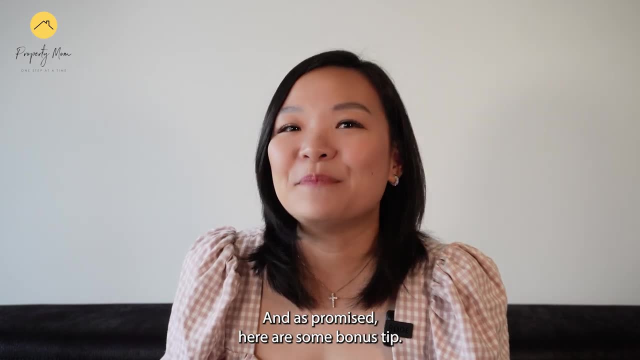 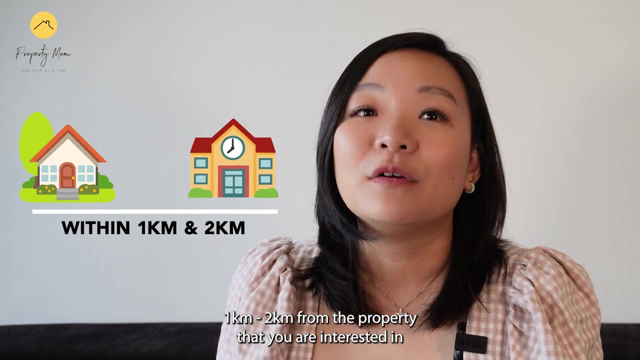 stay safe, chilli phan. a little bit more insight into the process, if you're still watching this video. thanks for staying with me and, as promised, here are some bonus tips. tip number one: if you want to see if your preferred primary school is within one to two km from the property that you are interested in. 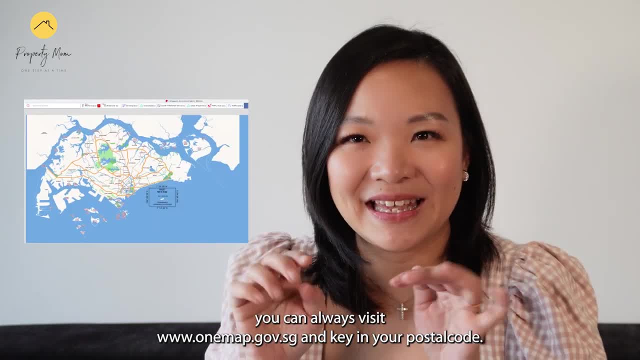 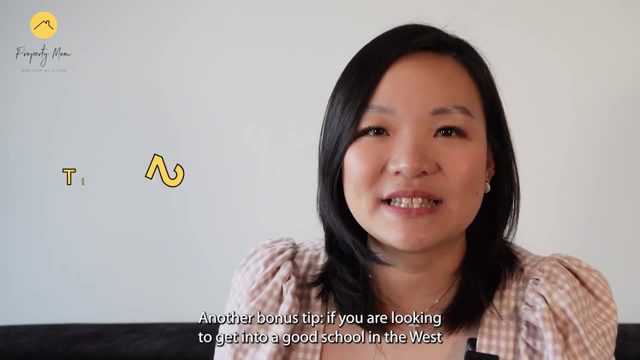 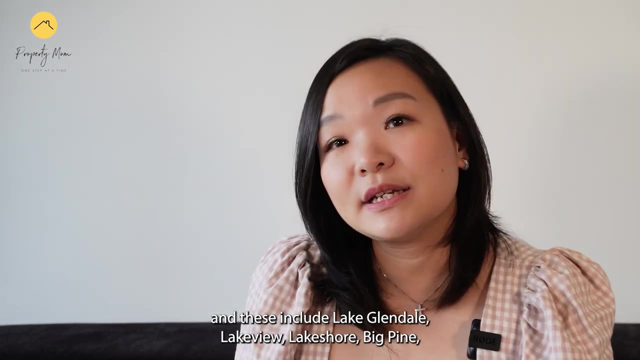 you can always visit onemadgov and key in your poster code. this will show you all the school available within one to two km. another bonus tip: if you're looking to get into good school in the west, there are some private properties around roland primary school and this includes.